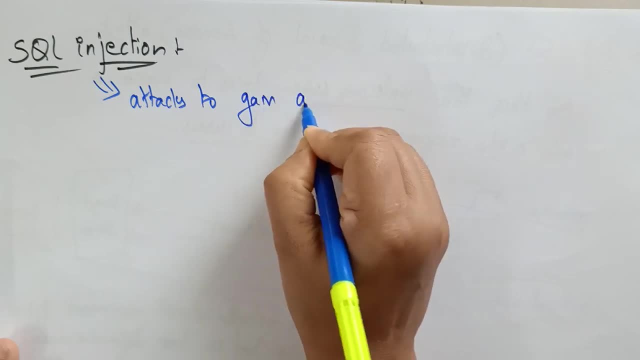 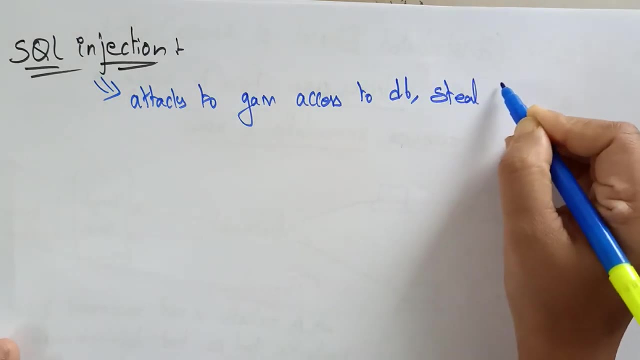 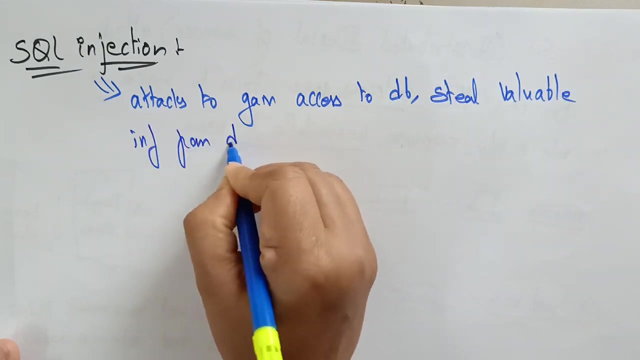 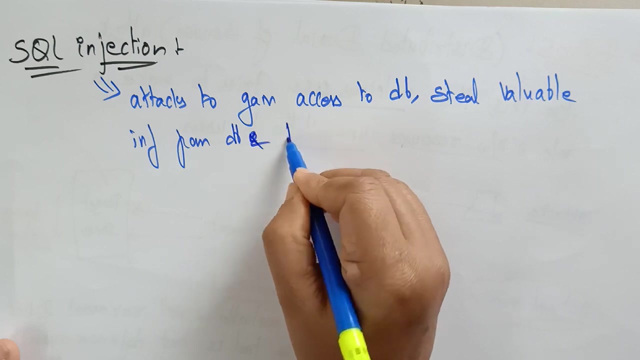 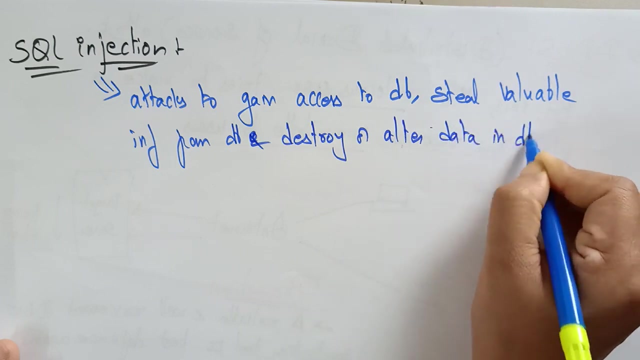 SQL injection attacks to gain Access to Database and steal What it is doing. it steal the valuable information, Steal the valuable information from database And even also destroying or alter The data in the database. So this is what this SQL injection will do. 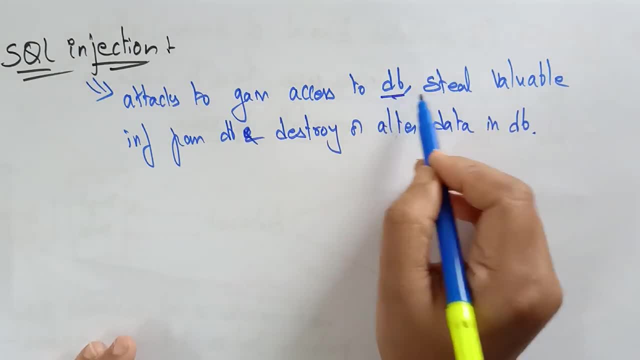 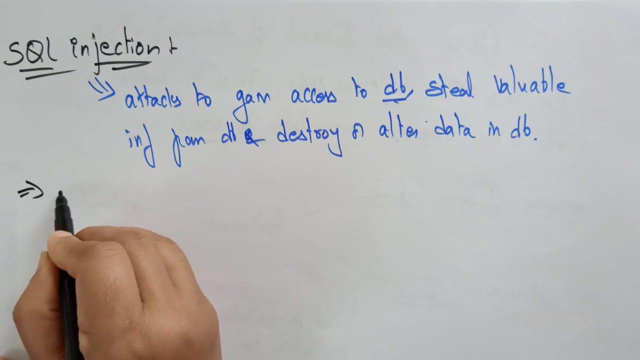 So the SQL injection attacks to gain access to the database and it is going to steal the valuable information from the database and it even also destroy or alter the data in the database. So the SQL injection actually occurs- How, let's tell. let me explain. 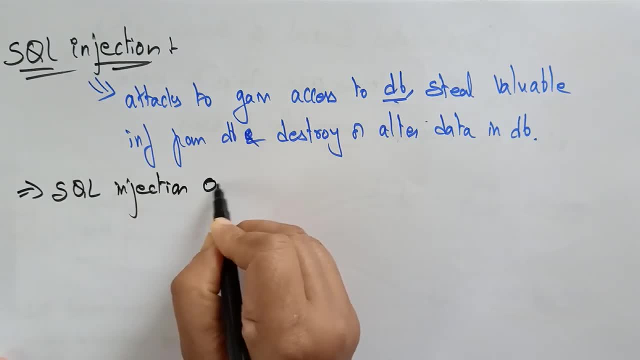 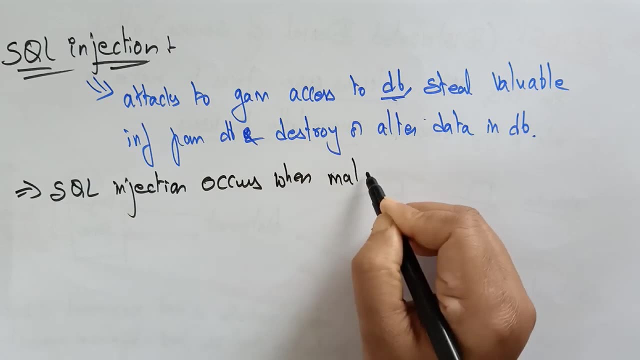 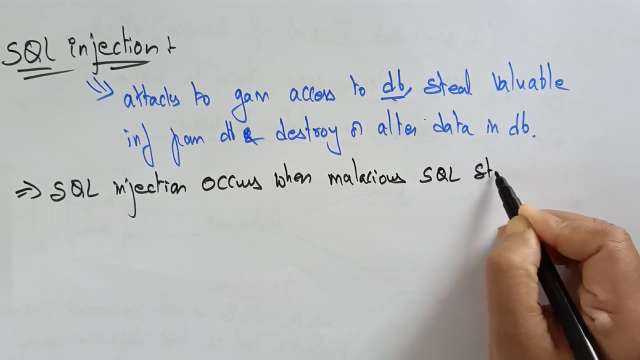 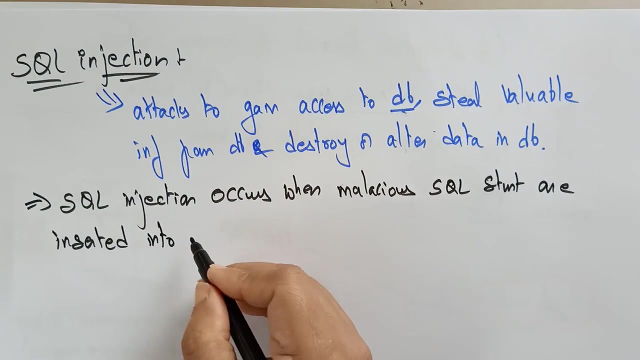 SQL injection Occurs when Malicious SQL statements means the unwanted statements- Okay, which is having some malicious code, Malicious SQL Statement or inserted, Or inserted into form fields. So when you're entering the data on the database where you are going to enter, 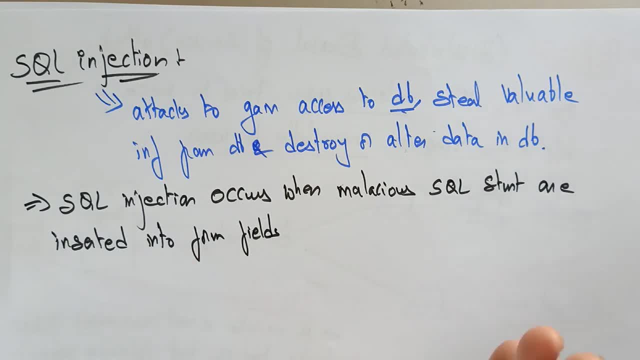 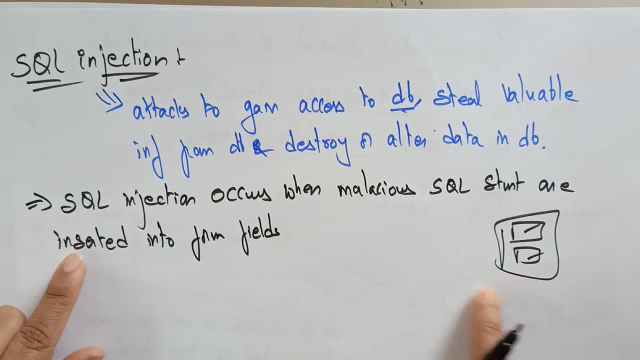 Usually we are entering the in the client side, We are entering the data on the form table. Okay, just like a form table, in the form table You are entering the data. So while you're entering the data, So the SQL injection occurs when the malicious SQL statements are inserted into the form fields. 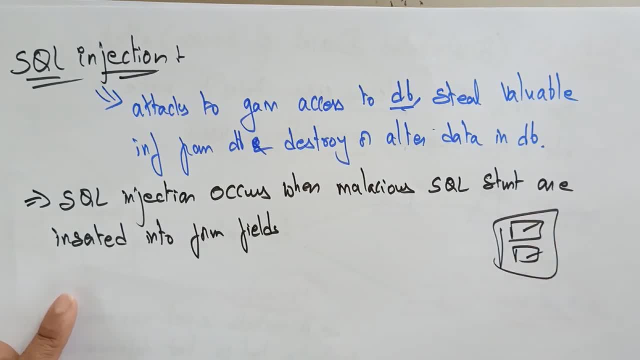 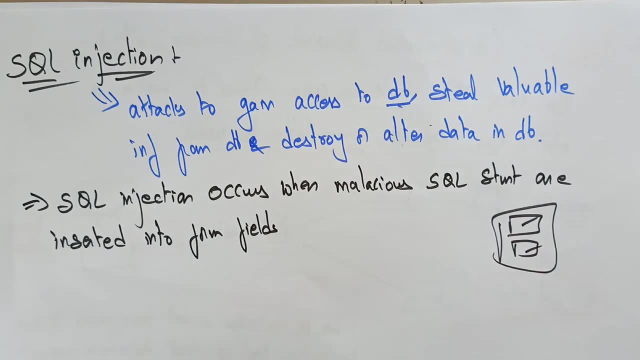 So in this form field, some malicious SQL statements is also inserting into this field along with the user. user field Okay, form fields So here which are not Properly protected in code. Okay, to try and gather the information from database, So with: 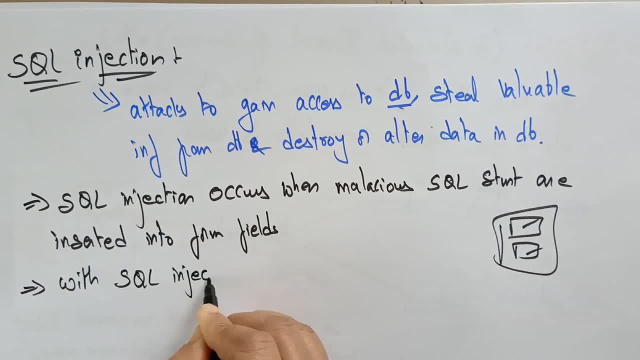 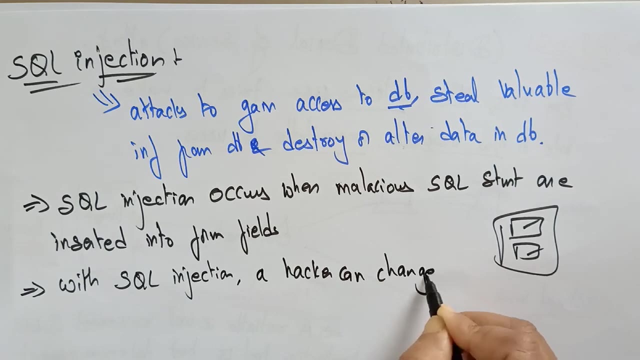 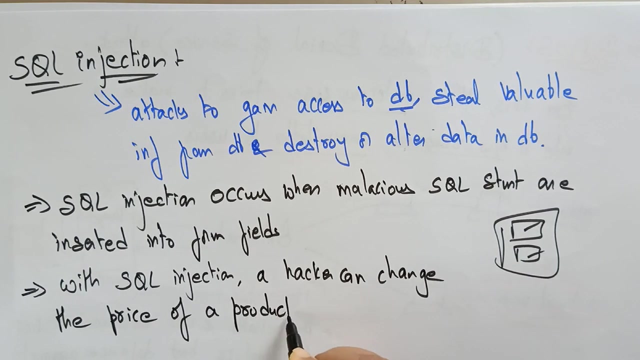 With SQL injection. So what a hacker will do with this SQL injection? So with SQL injection, a hacker can. Hacker Can- Change the Price of a product. He can. he can change the price of the product and gain the customer information. 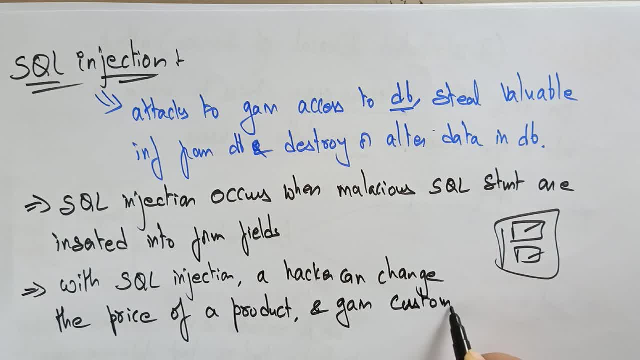 And gain Customer information. Okay, so this is what the SQL injection will do. So whenever we are, the hacker is trying to inject this some malicious code. That is what we call it a SQL injection. The hacker can change the price of the product. 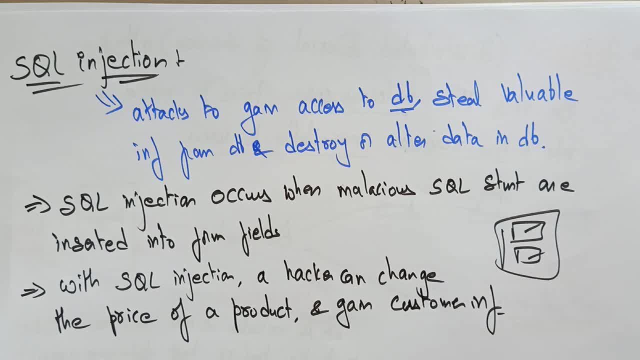 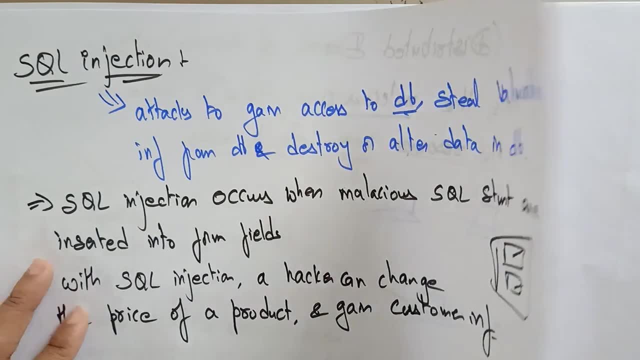 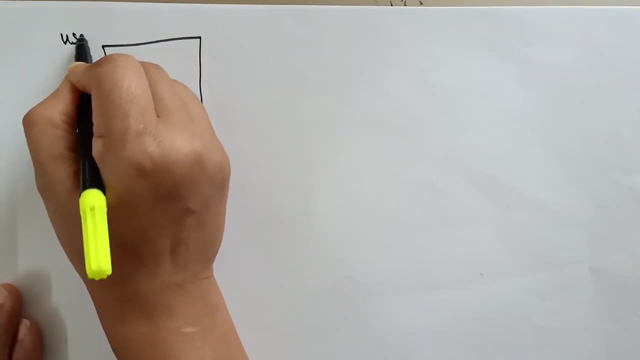 Whatever it is there in the database. This is one of the example. The pro Hacker can change the price of a product and he can gain the customer information Also. let me explain you with a simple example: SQL injection. So let's take this: is the user from user is there. 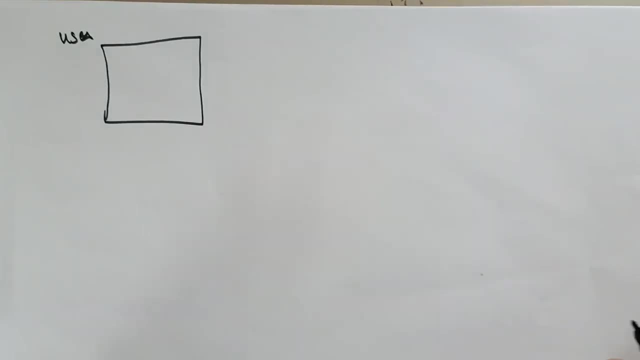 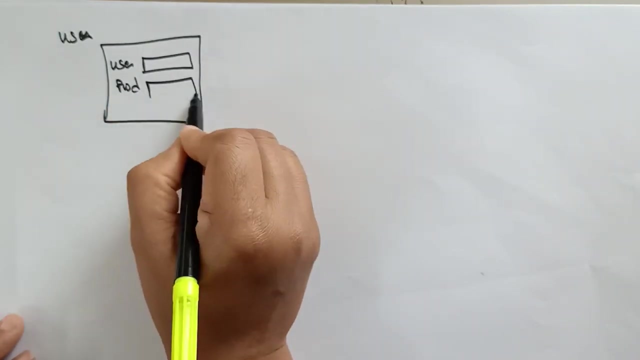 So user is entering that you want to access his database. So how you're going to access his database? by using the username and the password. So okay, username and the password. Okay, so he is entering with the password. Some conditions will be there. 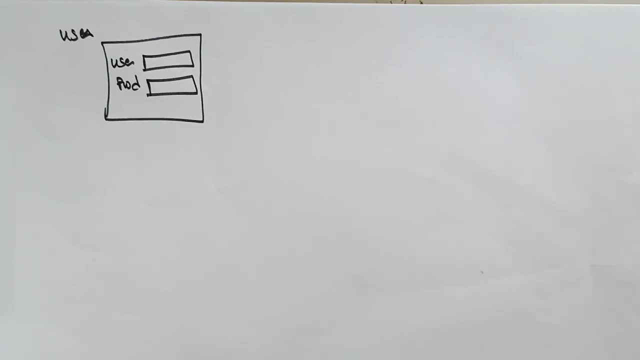 Like a: capital letters, small letters has to be included So that hacker can identify these things. Okay, This site is protected with some like: the password should be like this: like the: it includes the capital letters, small letters, like that It should. he has his identifying. 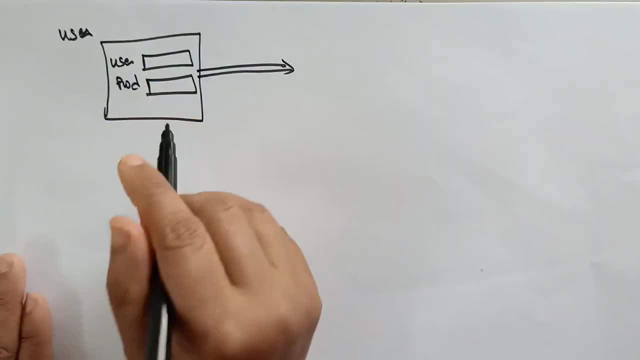 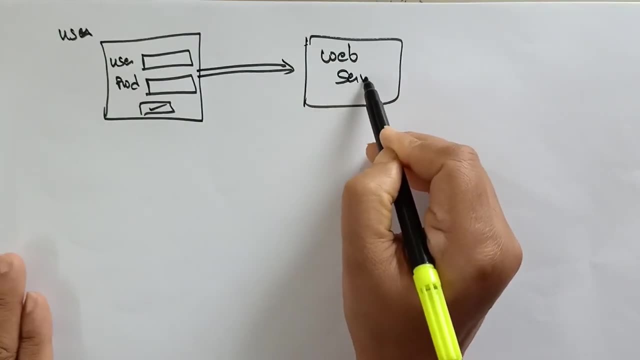 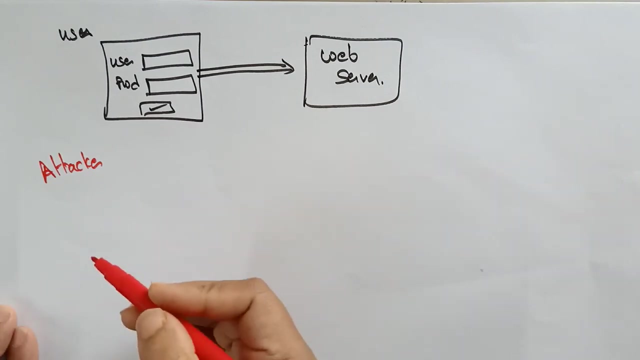 So the user, By entering the username and the password whenever you click on the submit, he is going to access the web server. Okay, is going to access the web server. Now that Attacker? that I got what he's doing. The attacker is doing the SQL injection. 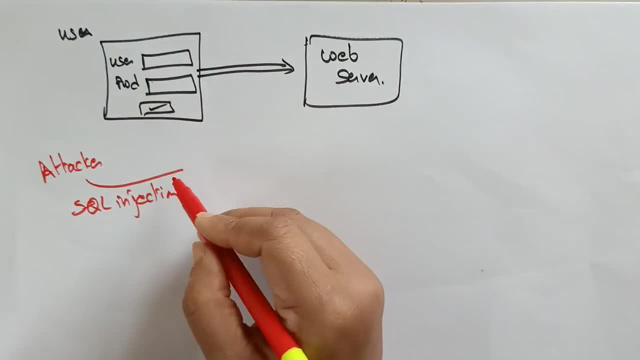 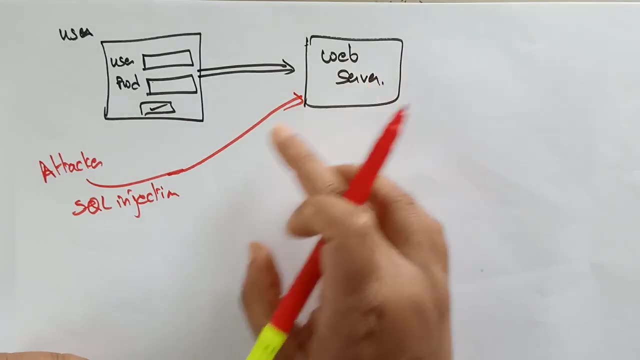 So, whatever the statement, he is there, it is in the password. Okay, so a malicious code is injected, a malicious code will be injected and he is trying to access the web server. So whenever he entered the malicious code, it is matching with these username and the password and he is trying to access a web server. 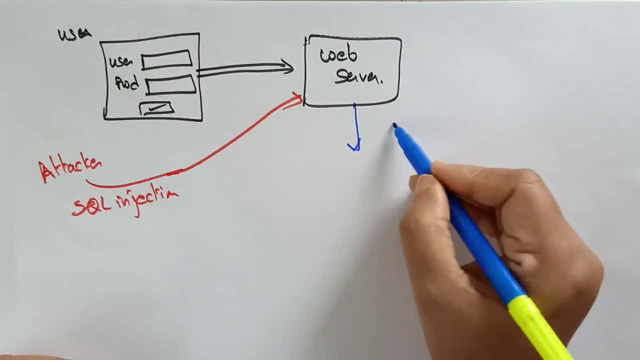 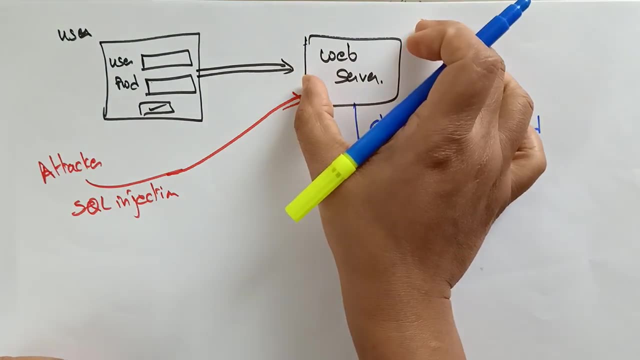 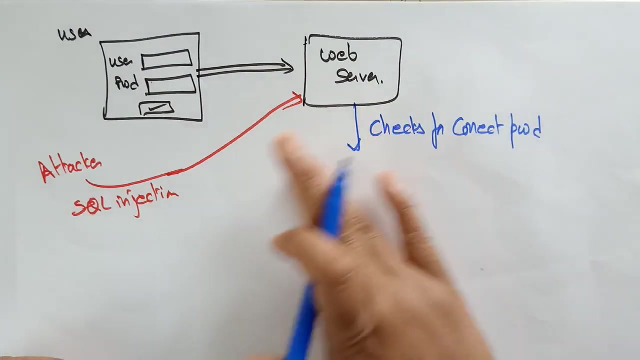 So whenever it he access the web server, Okay, The web server checks For correct password. He's is. the web server can't identify who is the person, means is the correct person or not He is, doesn't I? it doesn't bother about it is is just SQL. is injection along with this field? 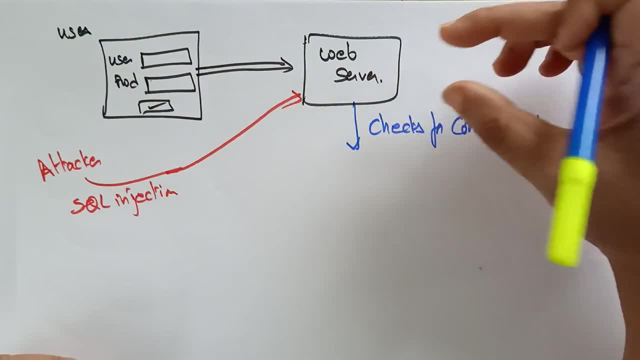 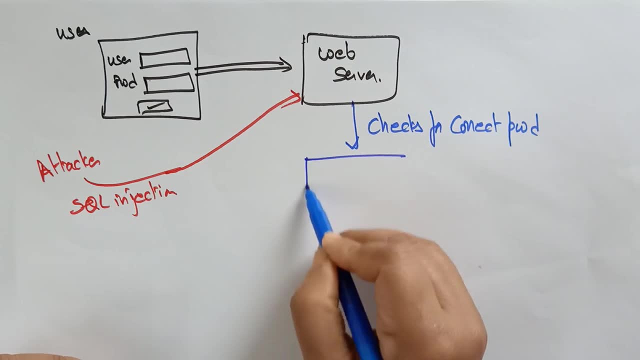 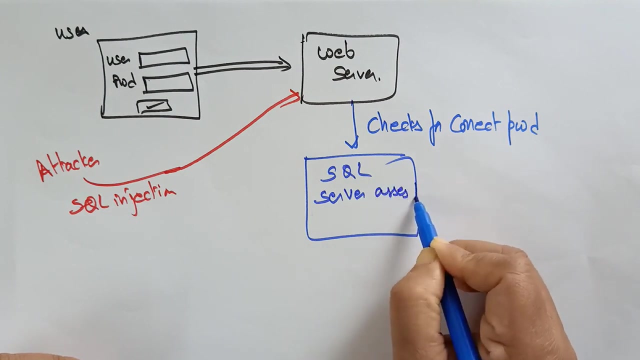 So he can't identify an attacker is also entering into the web server. So simply, whatever the users are there, He checks for the correct password and enter into the SQL server- that is a database SQL server as SSD true condition. So whatever he is going to access, that will be displayed. 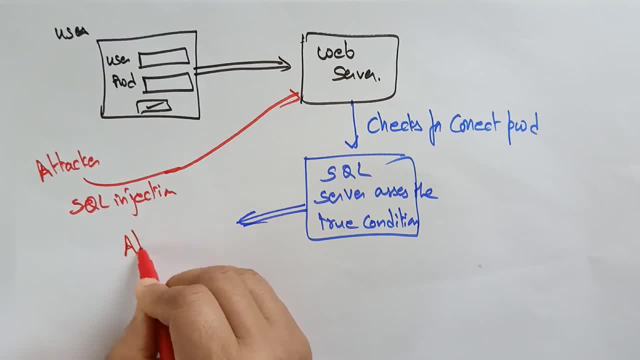 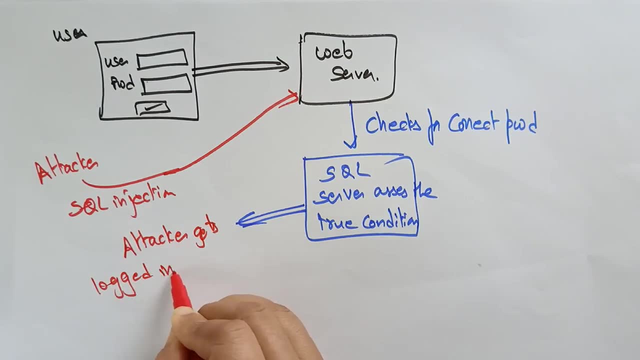 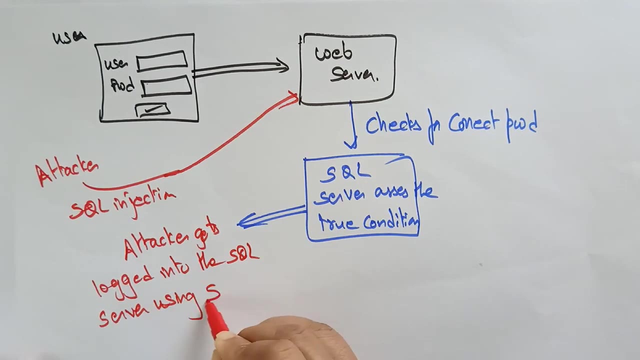 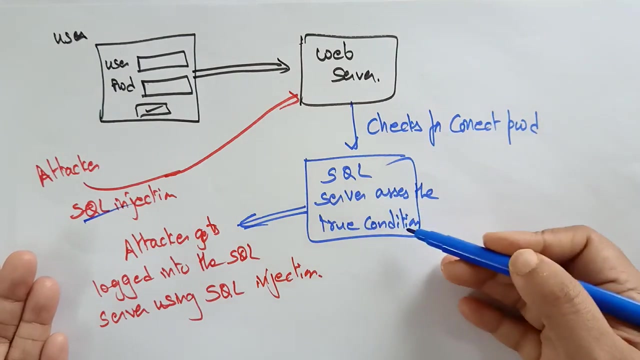 So that is display to whom that now the attackers Get logged into The SQL server Using SQL injection. Now the attacker can easily now, with the help of these SQL injection, He entered into the SQL server whenever he entered into the SQL server. 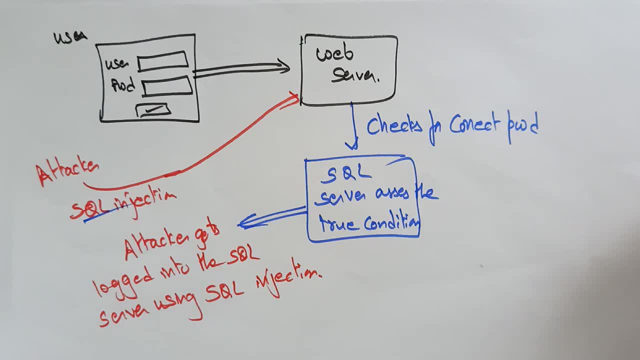 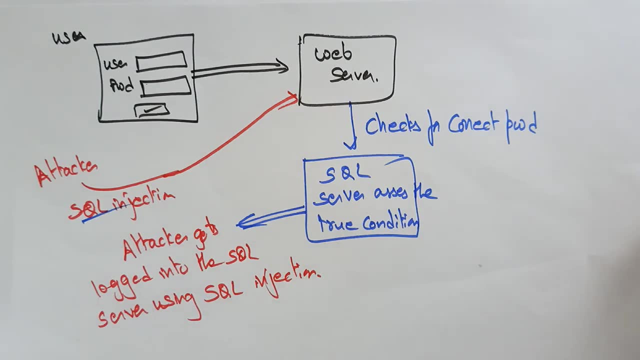 He can access the database, He can manipulate the database, He can modify that, he can change the details, He can gain complete information of the customer. Okay, so this is what the SQL injection attack was. So here the user as well as attacker is good. 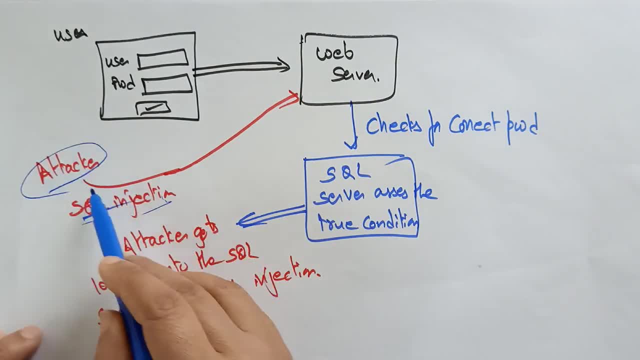 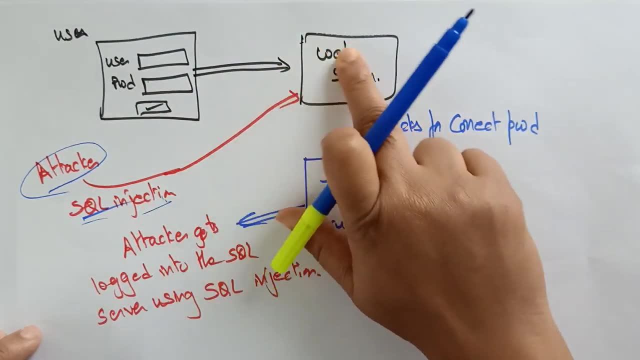 Both are going to access the web server. So how the attacker is going to access with the help of this information- Okay, the SQL. he is entering some code in this password along with this He entering into the web server. Now what is the prevention? 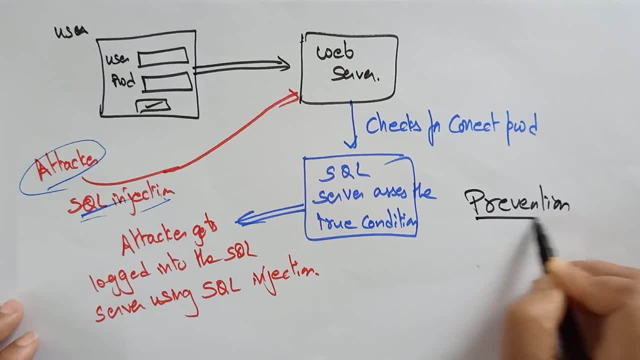 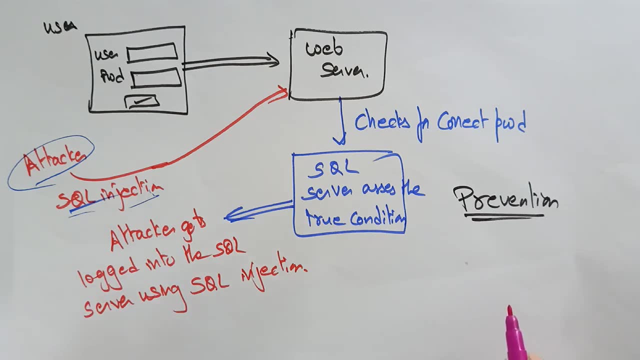 So this is happening. So this leads to some severe damage to the server as well as to the user information. Then how we are going to prevent this? the prevention for the SQL server is the only thing- is in order to keep your database secure. You should practice. 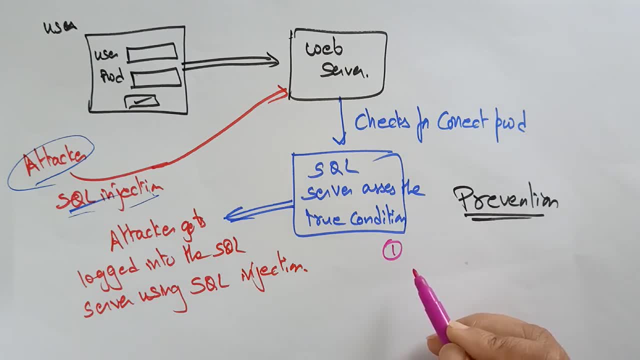 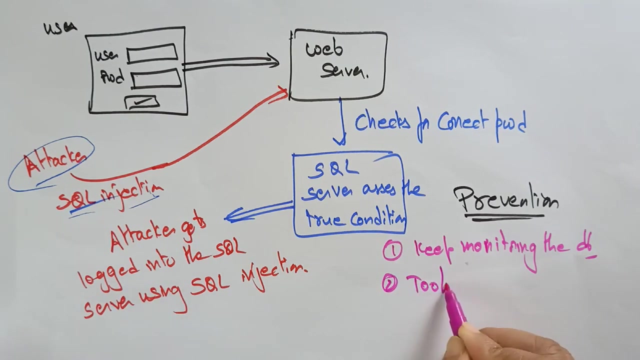 This regular auditing, remediation, Okay, of your application to ensure that any vulnerabilities discovered. Okay, so we have to keep monitoring, Monitoring the database, auditing your database and rechecking your database Every time you trip, keep monitoring the database and next you have to use some tools and software: tools and software to prevent this SQL injection.